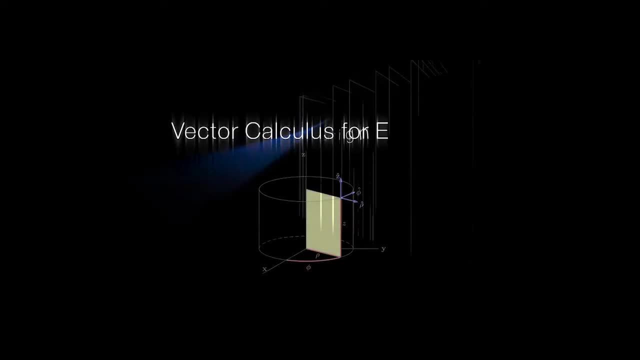 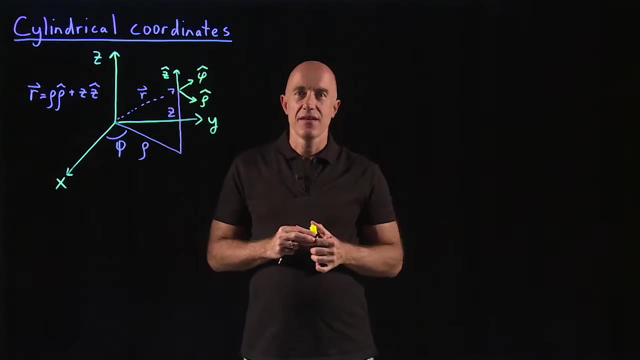 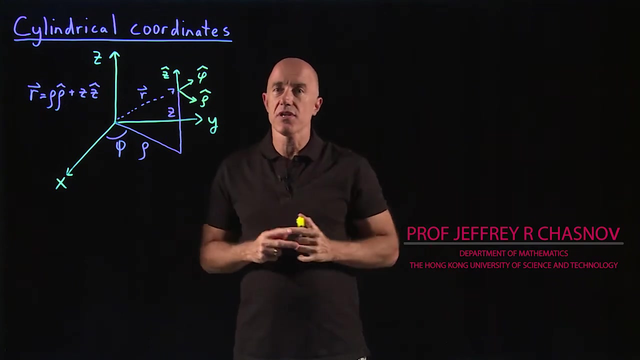 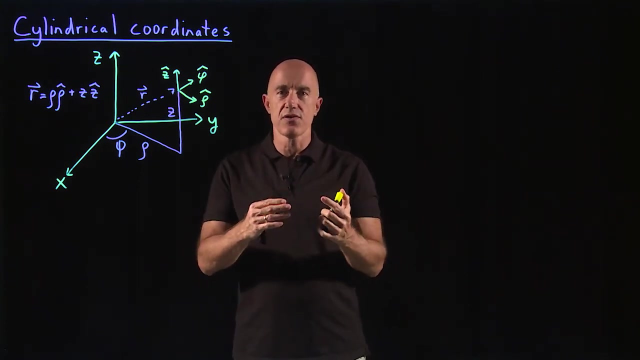 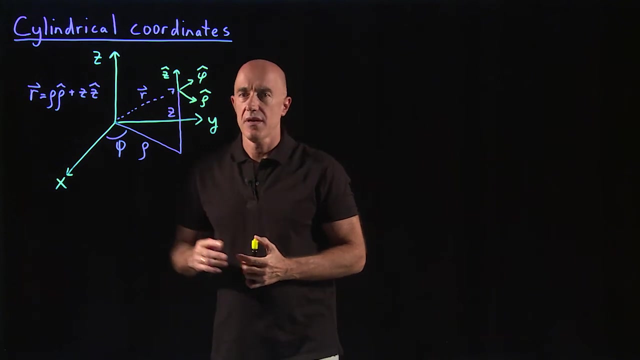 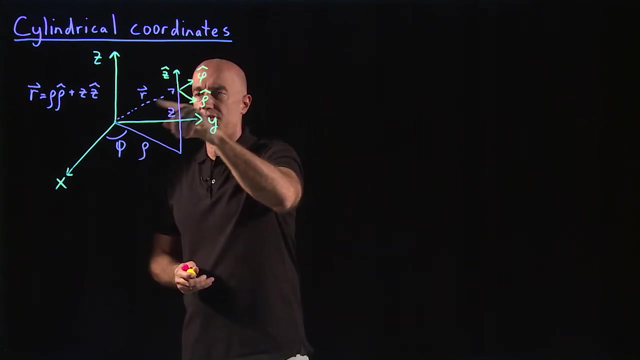 So we've already discussed polar coordinates. This is the two-dimensional circular type of geometry. A circle is a cross-section of a cylinder, So if you wanted to extend polar coordinates to the third dimension, it would be called cylindrical coordinates. So here I've shown you a graphical representation of cylindrical coordinates. This is the position. 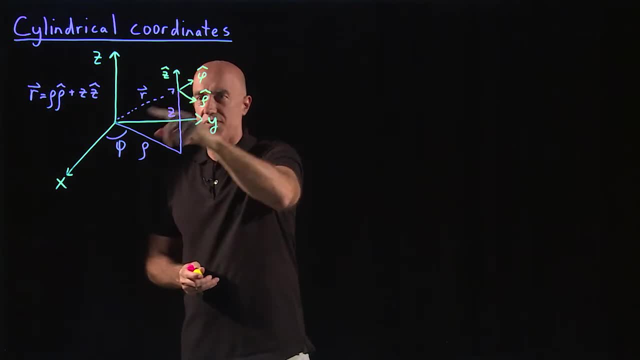 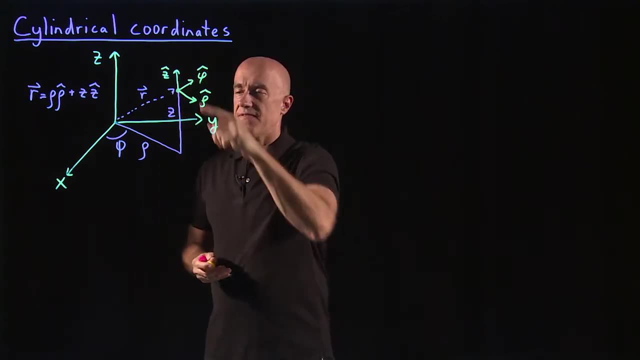 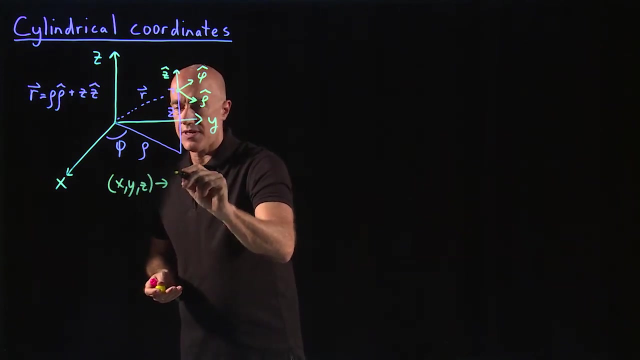 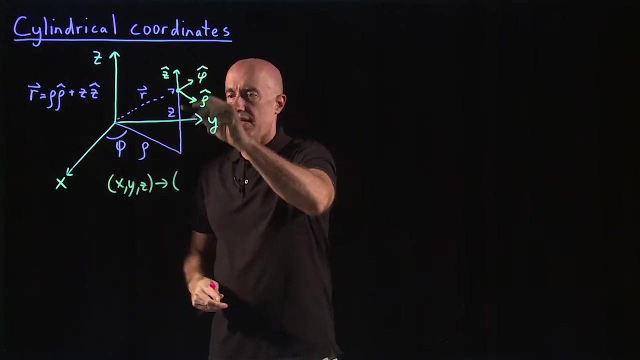 vector. It's not that straight, but it's the position vector pointing to this point here. Then we can identify the x, y, z coordinate of that point Using three different variables. here would be rho, which is the length If you project. 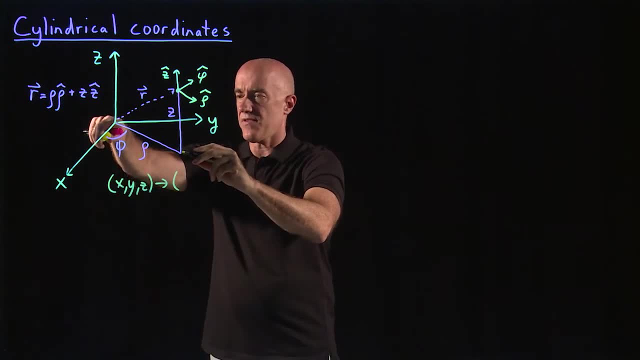 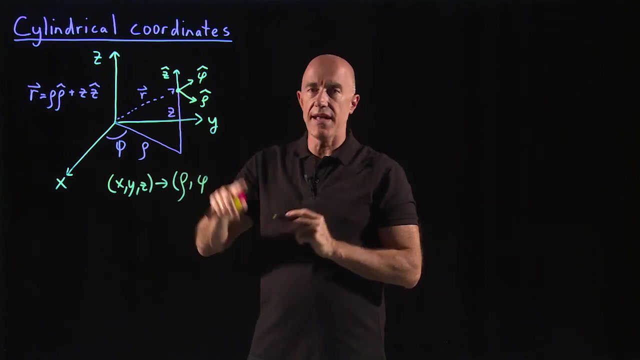 that point onto the x? y plane. it's the length from the origin to the projection on the x? y plane, And then the angle that projection makes with the x-axis is phi. In polar coordinates we call that this r and theta because that's kind of the standard in two dimensions. 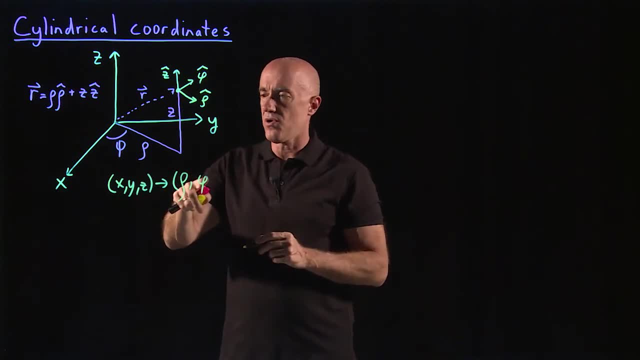 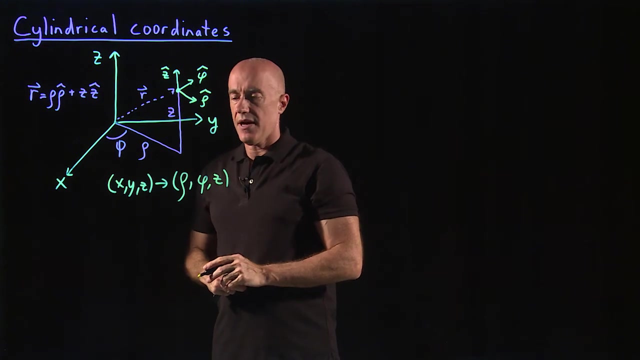 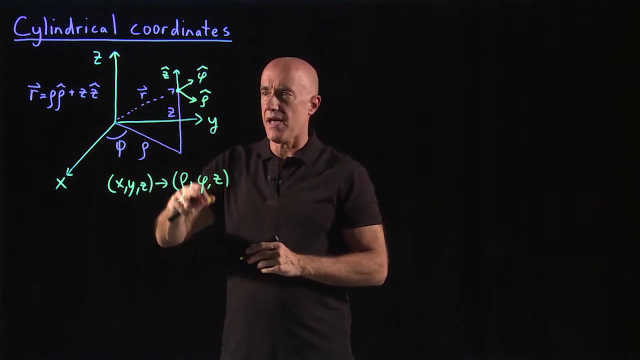 When we go to three dimensions. now we're calling this rho and phi, And then the third coordinate is z, the vertical height above the x- y plane, And that specifies this coordinate. So this is actually. this is just polar coordinates. Instead of r, theta, we use rho, phi, Polar. 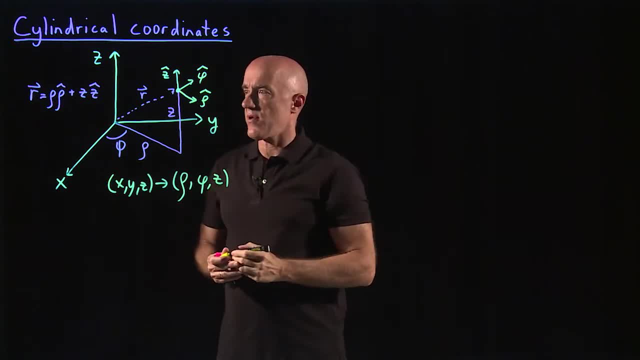 coordinates expanded into the third direction. The position vector then is written as rho times rho hat. So rho hat is the unit vector in the direction of rho plus z times z hat. z hat was our k in Cartesian coordinates. And the third unit vector then is phi hat, which is in the direction of increasing phi. 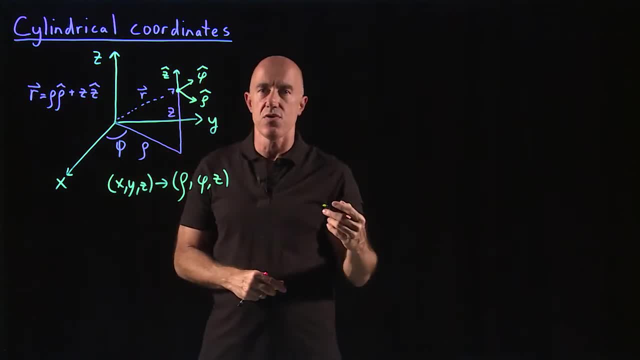 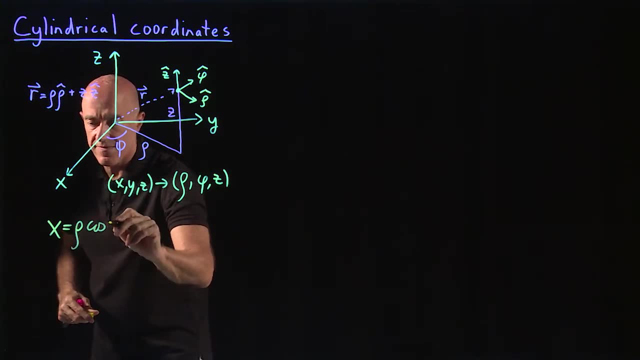 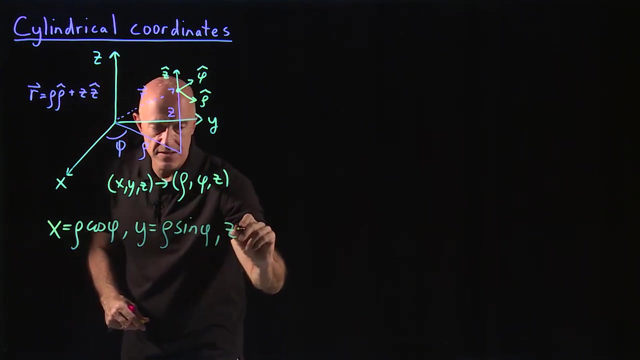 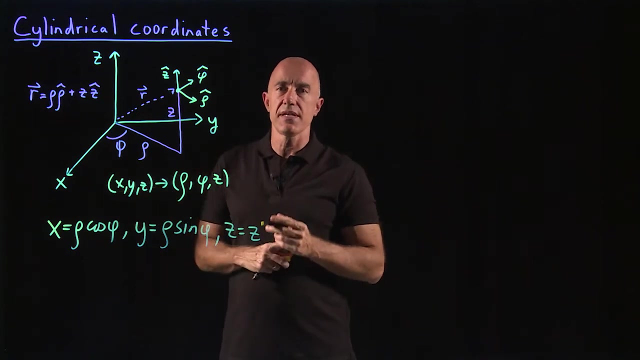 So the change of variables formula from Cartesian coordinates to cylindrical coordinates is: x equals rho cosine phi, y equals rho sine phi And z still is the Cartesian coordinate, z. You can compute the Jacobian here to get the change of the dx dy volume element. a change. 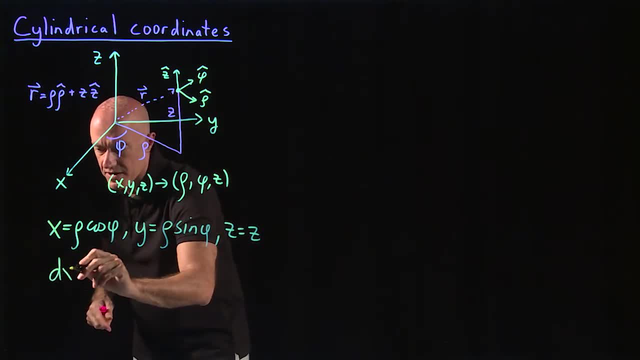 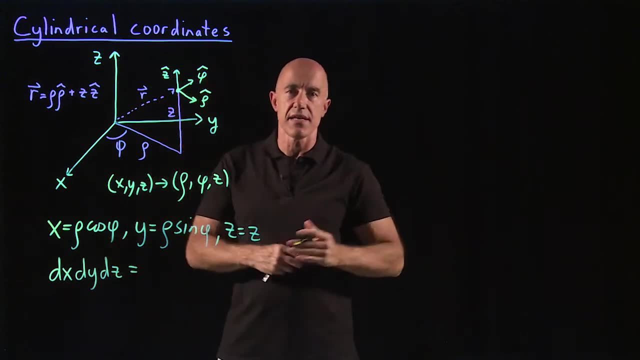 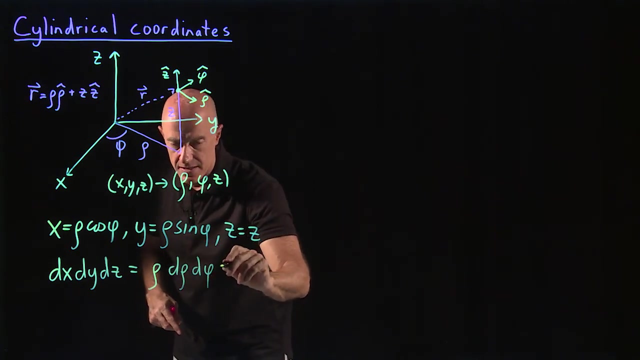 of variable, And then you can do this formula, And if you do that as part of your problems, you get dx dy dz. Well, it's actually. we did it already. for polar coordinates It would just be rho d, rho d phi dz, because the z coordinate doesn't add anything to this. 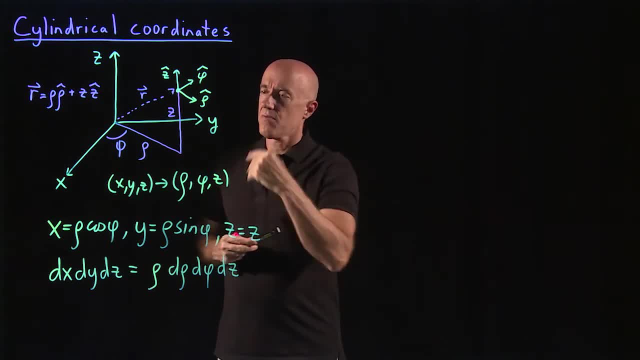 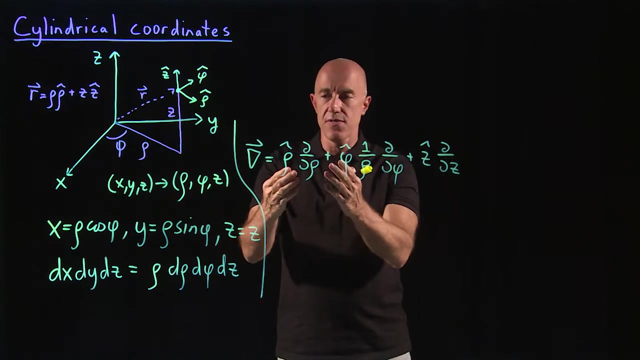 OK, We need the differential operators in cylindrical coordinates, So we're going to go to a distribution did and let me please help. So here we have a dependent response. Once again, this is a geometric equation, So we're going to use some просто visto curves. 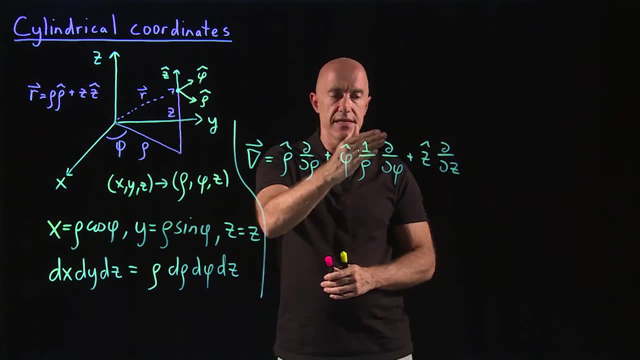 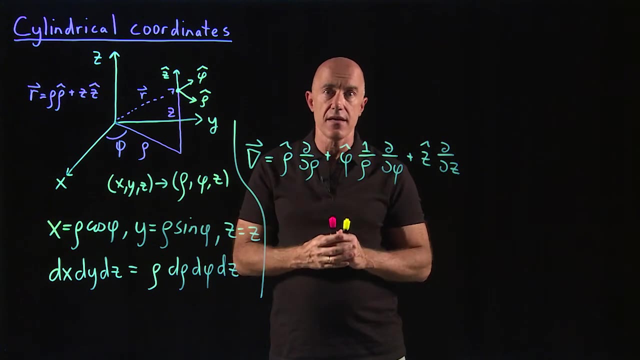 走 to explain thisavas과 The along vou diz is the differential coefficients over rho, dd, phi plus z hat, ddz. So there's this extra factor of 1 over rho. Remember that both rho hat and phi hat are functions of phi. 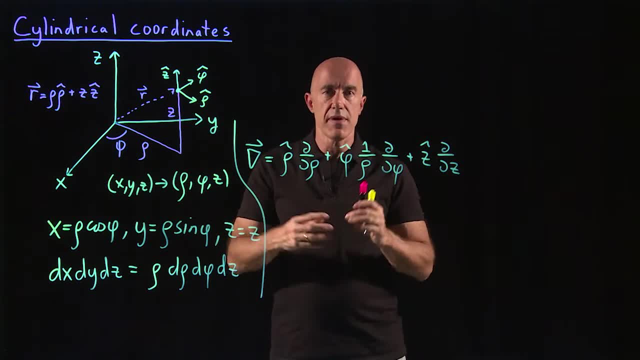 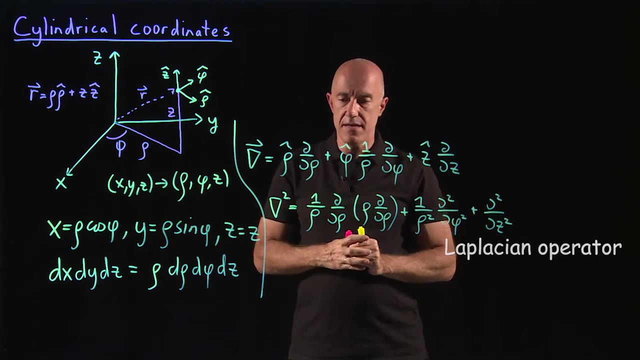 So when you differentiate, you always have to make sure you differentiate the unit vectors. OK, let's look at the Laplacian now. OK, so this is the Laplacian operator, a bit more complicated. 1 over rho dd rho of rho dd rho. 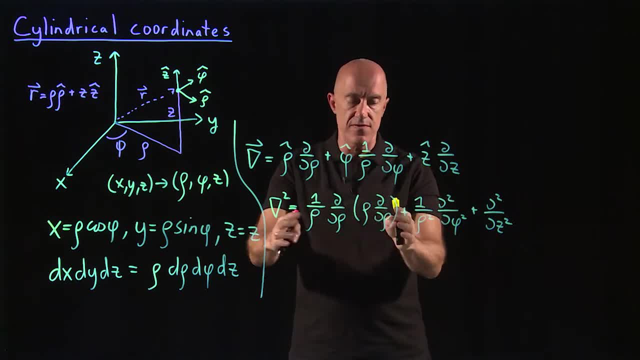 So this has both a first derivative in it and a second derivative in it, plus 1 over rho squared d squared, d phi squared, and then plus d squared dz squared, because the z unit vector is fixed, doesn't depend on phi. So if you wanted to solve a PDE, that 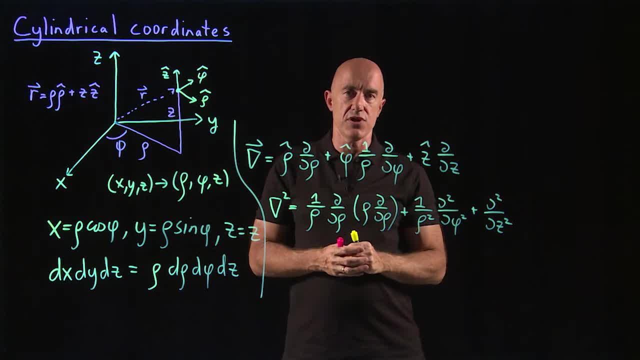 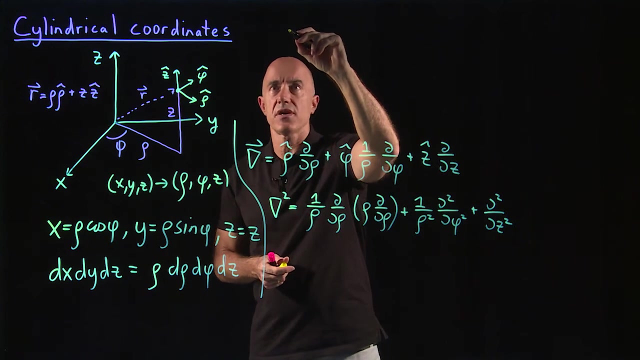 has some sort of cylindrical geometry associated with it, such as the electromagnetic field inside a cylinder cavity, then you would need this form of the Laplacian. OK, now let's look at what do you do if you have a vector. so a vector a. 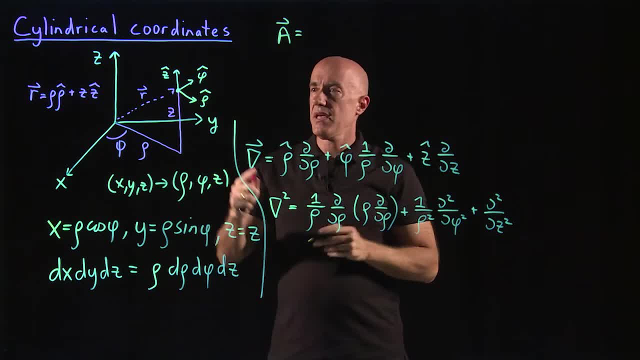 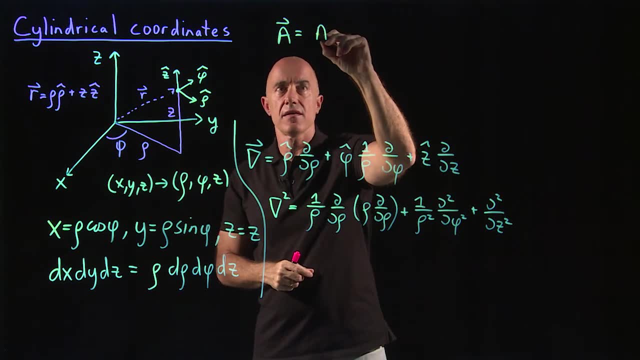 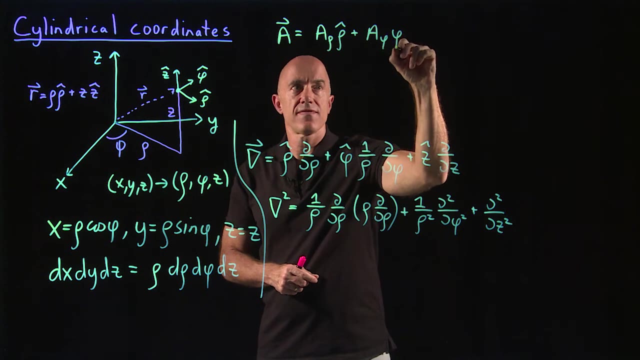 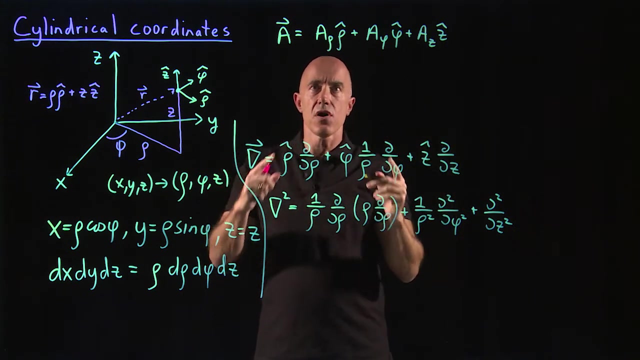 say, A has components in the rho direction, the phi direction and the z direction. So I'll write that as a rho times rho hat plus a phi times phi hat plus a z times z hat. So a rho is a function of rho, phi and z. 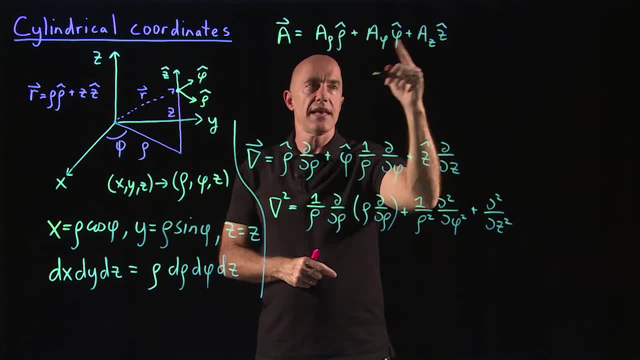 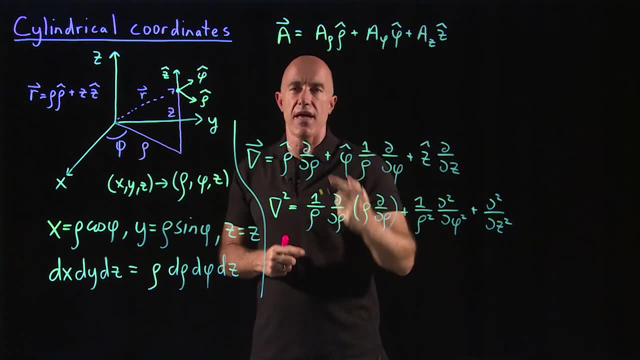 A phi is a function of rho phi and z, And a? z is a function of rho phi and z. So now I want to talk about what is the divergence of a in cylindrical coordinates and what is the curl of a in cylindrical coordinates. 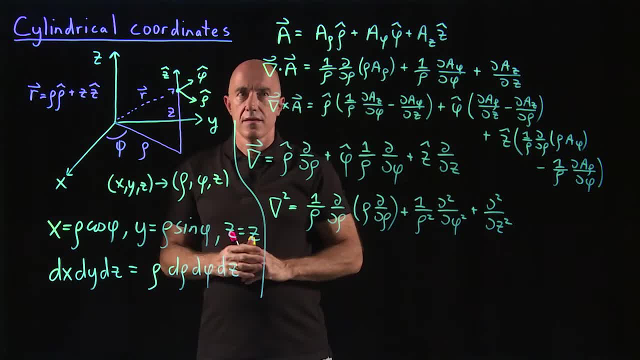 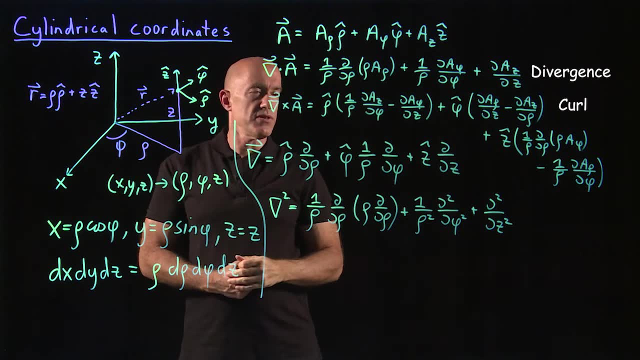 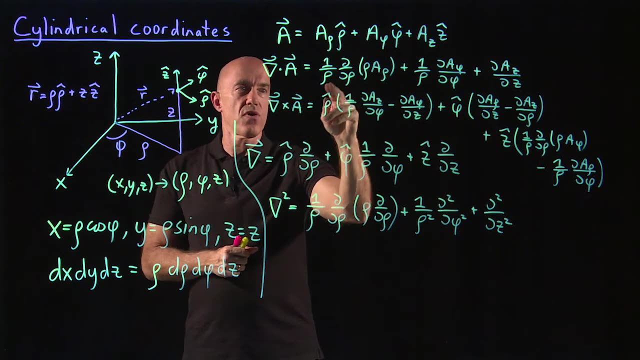 So let's have a look at that. OK, so this is the divergence of a and this is the curl of a. You see how the expressions are quickly becoming complicated. So the divergence of a is 1 over rho d d rho rho times. 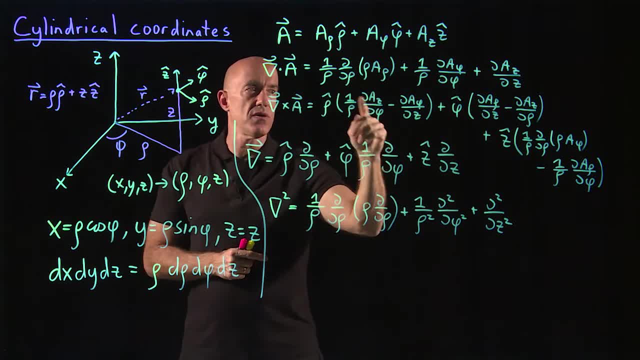 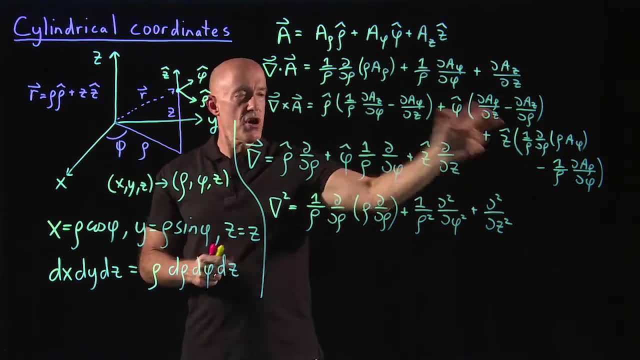 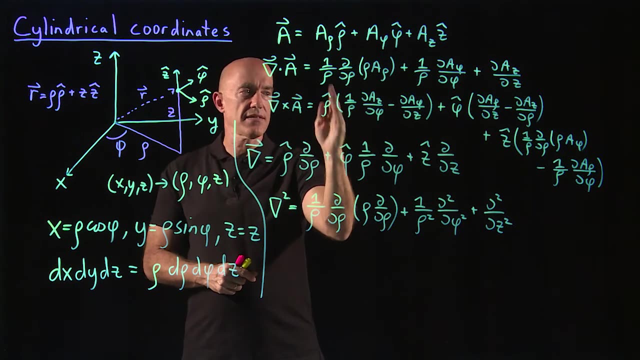 the component of a along the rho hat direction a rho plus 1 over rho d a phi d phi plus d a z d z. The curl is more complicated, So the del cross a the component in the rho hat direction is 1 over rho d a z d phi plus 1 over rho d a z d z. 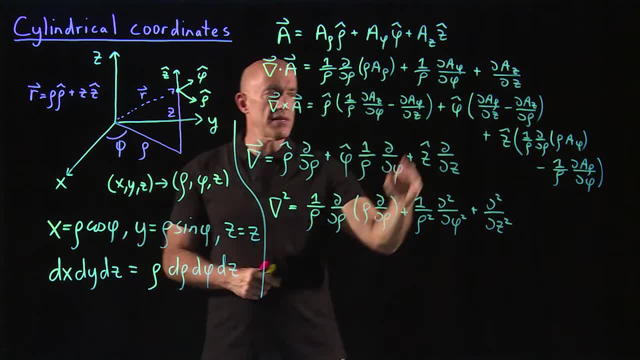 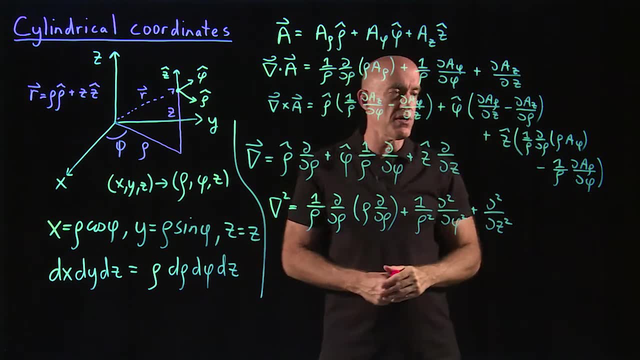 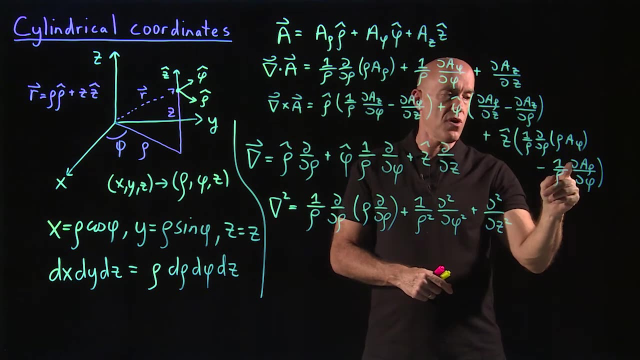 d phi minus d a phi d z plus. the component in the phi hat direction is d a rho d z minus d a z d rho plus. the component in the z hat direction is 1 over rho d d rho. rho a phi minus 1 over rho d a rho d phi. 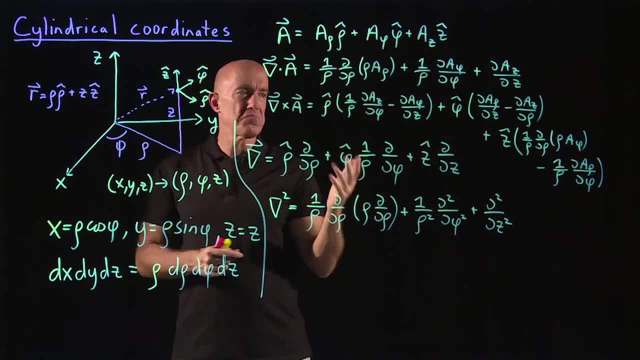 OK, quite complicated. So I'm capable of deriving these things, but I wouldn't want to. They're very messy. They're in the textbooks When you need them, when you're solving a problem that has a curl of a vector field or a divergence of a vector.